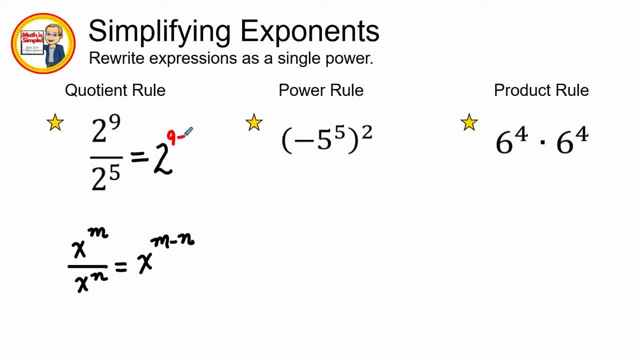 The exponent in the numerator is 9, and we are going to subtract it with the exponent in the denominator, which is 5.. So when we simplify further, in our final simplification we keep our base as 2, and 9 minus 5 is 4.. 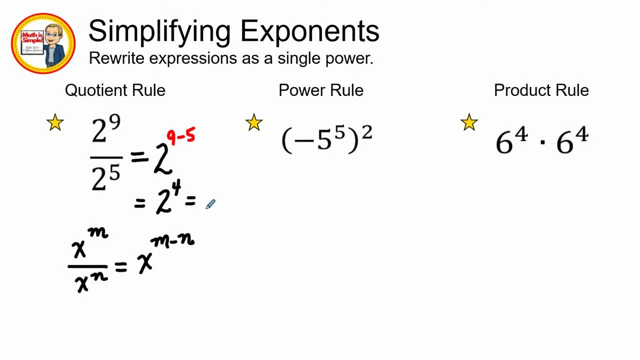 Now we can simplify, as I said, or simplify just a little bit more: 2 times 2 is 4, times 2 more is 8, times 2 more is 16.. So, fully simplified, the correct answer of 2 to the 9th power divided by 2 to the 5th power equals 16.. 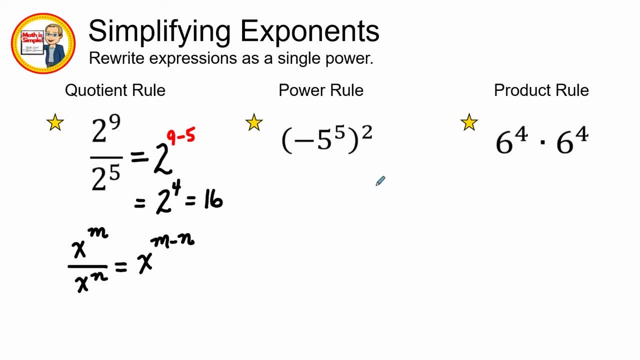 Now let's move over to the power rule, And one main thing that we learned in the power rule is that we're going to multiply our exponents, And in this case, the exponent on the outside, which is 2, gets multiplied with the exponent on the inside, which is 5.. 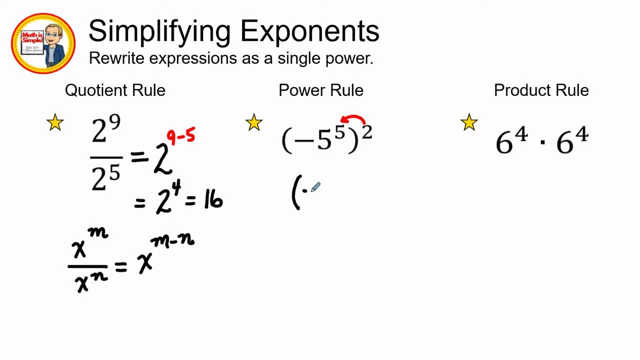 So if we look at negative 5, we're going to keep our base here And we're going to multiply these two exponents together Gives me 10.. Now I could rewrite it without the parentheses: and negative 5 to the 10th power. 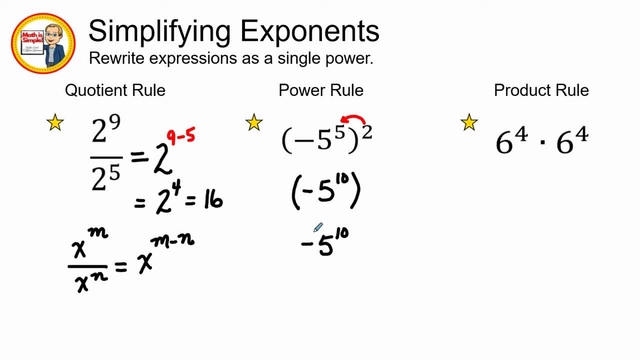 When we simplify this further, we want to make sure that we keep the negative 5 together. We don't want to use 5 to the 10th power and just tack a negative to the answer. Remember that any time that we have a negative number. 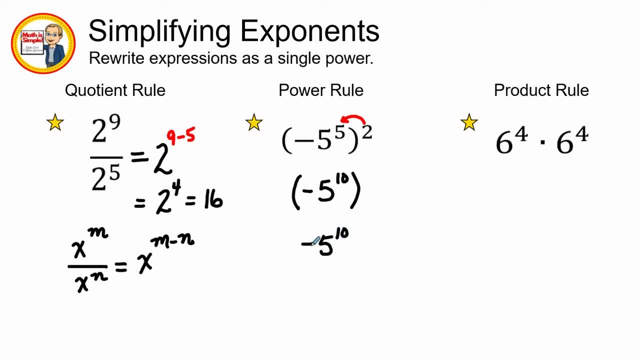 raised to an even number exponent, we are going to have a positive result. If I have a negative base and it's raised to an odd number exponent, we are going to have a negative answer, And that is because a negative and a negative is a positive. 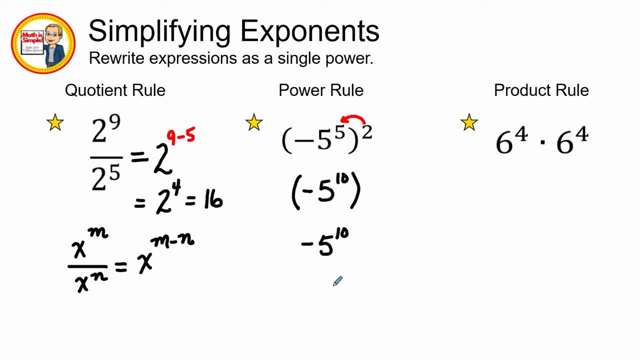 So two negatives multiplied together will give me a positive. Three negatives will give me a negative in my answer. So that's just a little Little tidbit right there. But remember, when we're doing the power rule we are going to be multiplying these two together. 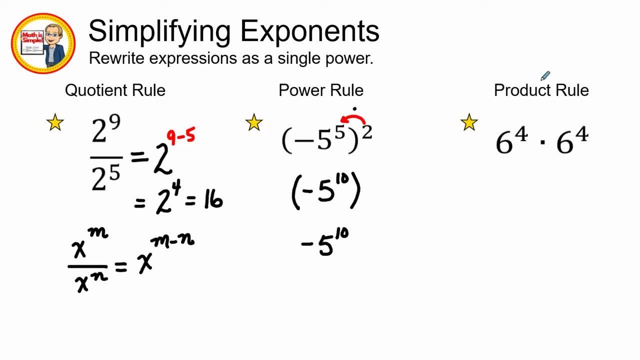 I'm going to put a point there to remind you to multiply. Now, looking at our product rule. The product rule is: when we have our base, and we have the base m with an exponent m, then we have our base x multiplied with x to the nth power.